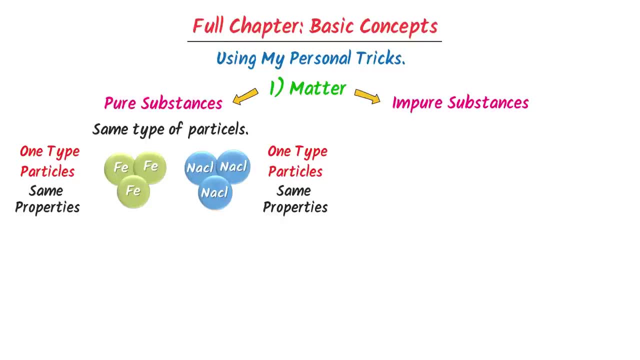 a pure substance. Here let me teach you one exam question: Why elements and compounds are called pure substances. Well, the answer is simple. They both are made up of one type of particles. So we say that elements and compounds are pure substances. For example: 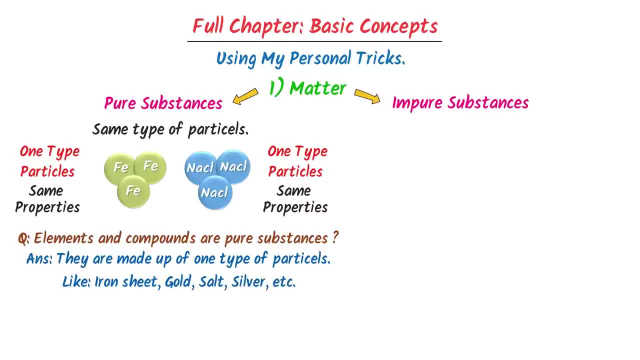 like iron, sheet gold, sodium, chloride, silver, etc. On the other hand, impure substances are those substances which contain different types of particles. For example, consider salt solution and salad. We can see that salt solution contains two types of particles. Secondly, 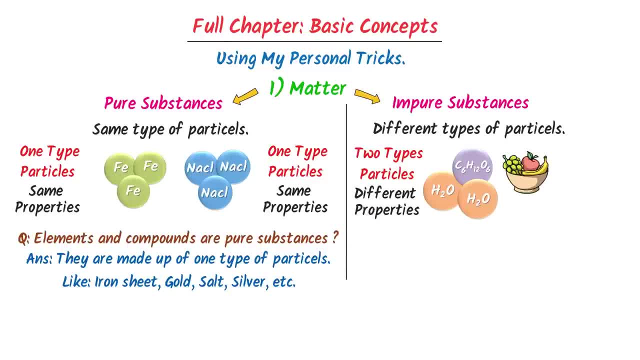 they have different properties. So we say that salt solution is impure substance. On the other hand, we can see that in salad there are more than two types of particles, and these particles have different properties. So we also say that salad is impure substance. Here let me teach you one. 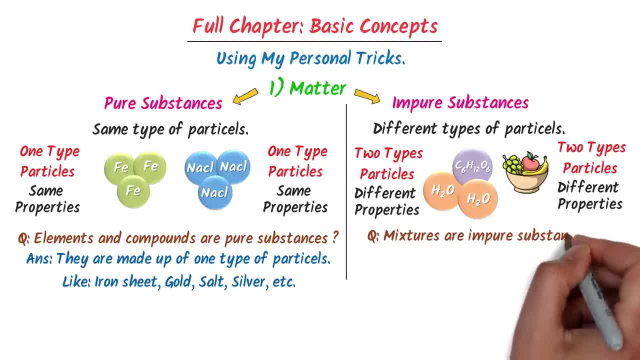 another exam question: Why mixtures are called impure substances. Well, mixtures are called impure substances because they are made up of different types of particles. Remember the name of these important mixtures, like air, seawater solutions, suspensions, colloids and alloy-like. 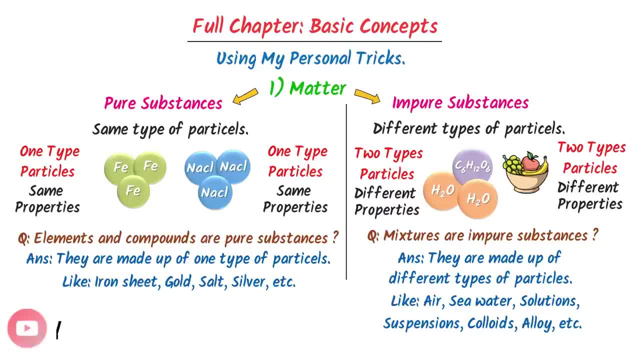 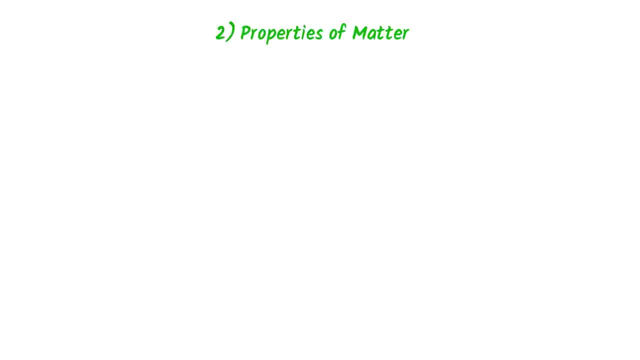 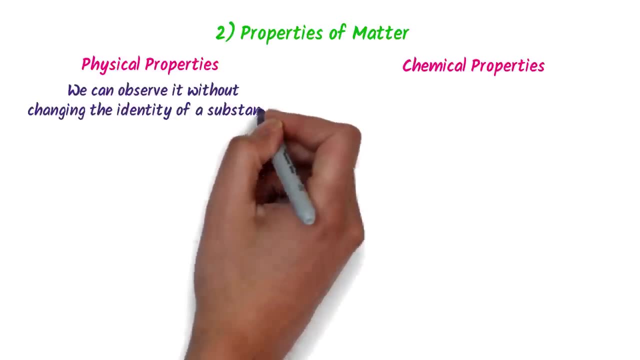 steel, which are usually asked in MCQs. So remember about pure substances and impure substances. The second topic is properties of matter. like physical properties and chemical properties, We can easily observe physical properties without changing the identity of a substance. Now, how we can remember the physical properties of matter? Well, I always use my 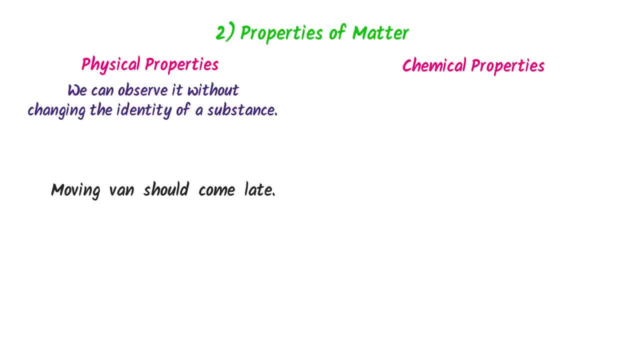 personal trick: Moving when should come late. Here, m stands for mass, v stands for volume, s stands for shape, c stands for color, l stands for length. Also, remember that all physical changes, such as point evaporation, sublimation and condensation, are physical properties. We can 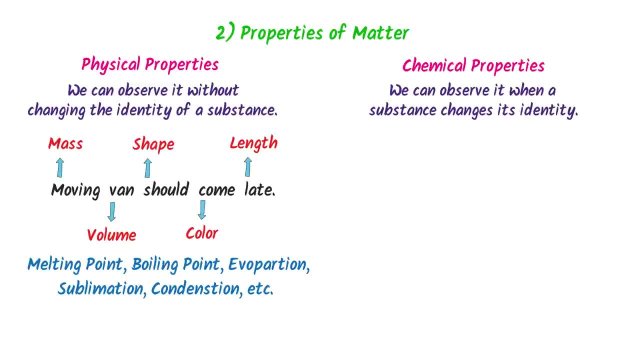 observe chemical properties when a substance changes its state. Now, how can we remember chemical properties? Well, we say that moving when should come late. In case of chemical property, we say that amir bai will come Here. a stands for acid, this s stands for air, b stands for base. 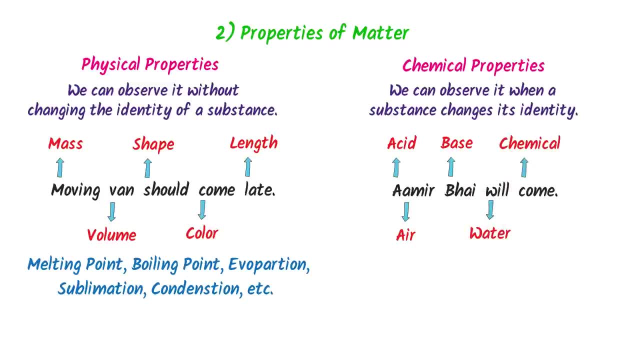 c stands for water, c stands for chemical. So a reaction of acid, reaction of air, reaction of base, reaction of water and reaction of chemicals all possesses chemical properties. Thus noted down, physical properties and chemical properties. Now let me teach you the third topic: physical. 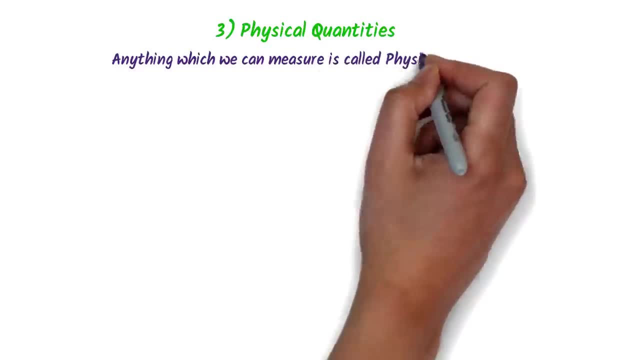 quantities. Well, anything which we can measure is called physical quantity. For example, consider 12 kilometer or 10 kilometers. Now let me give you a little more information in terms of physical quantities, For example. for example, consider 12 kilometers or 10 kilometers. Now you can measure. 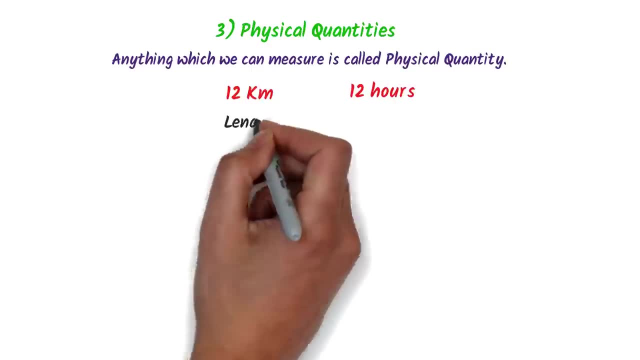 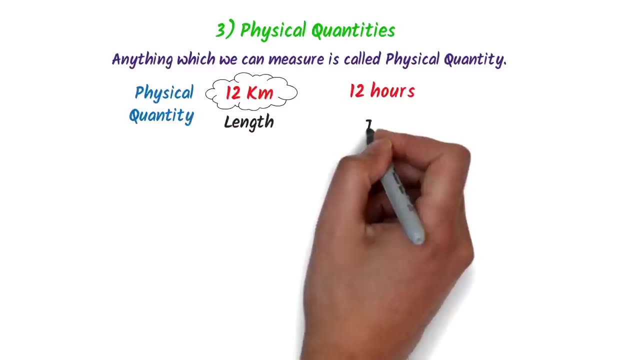 12 hours. Here we can measure the length of anything like 12 km, so length is a physical quantity. Similarly we can also measure the time like 12 hours, so time is a physical quantity. This topic is divided into three subtopics, like base physical quantities derived. 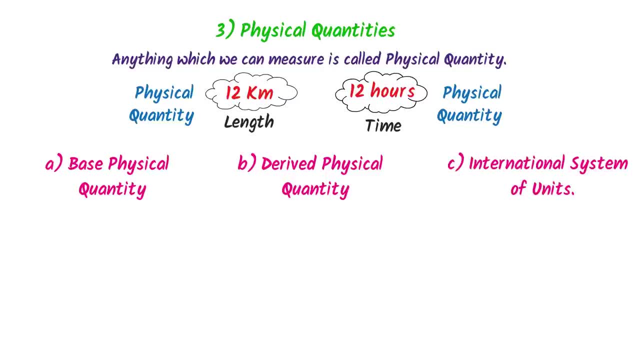 physical quantities- international system of units. Now, what are base physical quantities? Well, the seven physical quantities and terms of which other physical quantities are expressed are called base physical quantities, like length time. Secondly, those physical quantities which we can derive from the base physical quantities are called derived physical quantities. 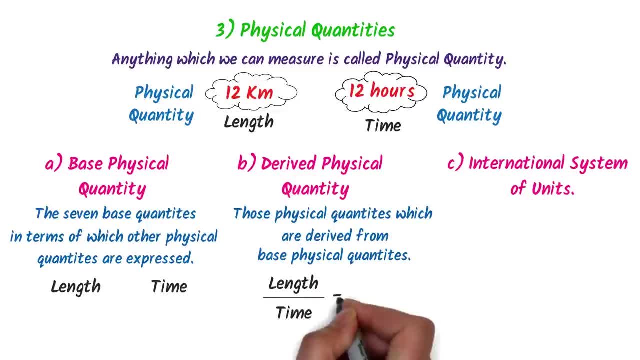 For example, when we divide length by time, we get speed. Here we know that length is speed and time. they both are base physical quantities. but dividing them we get another physical quantity, like speed, which is known as derived physical quantity. Now what is? 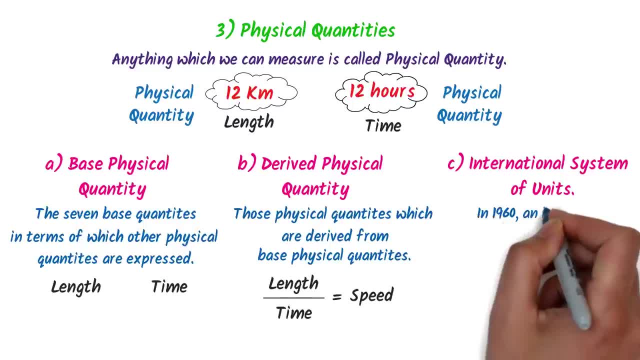 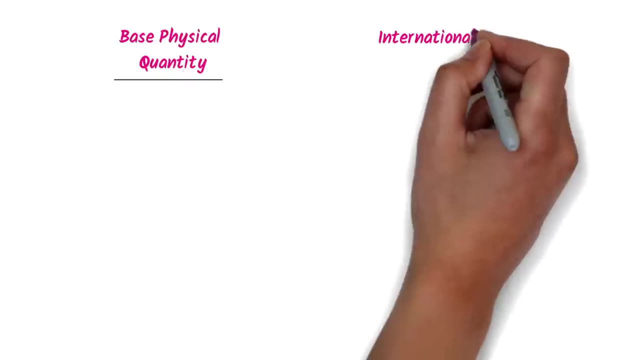 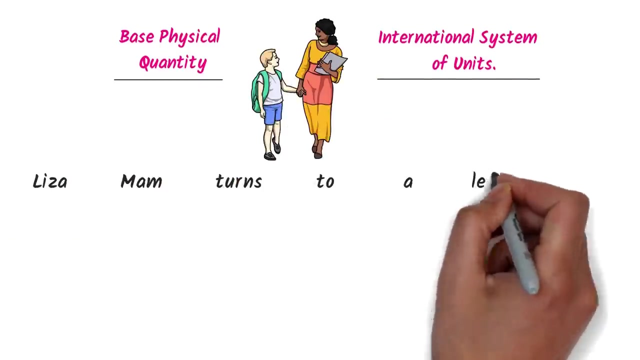 international system of units. Well, in 1960, an international system of units were established for seven base physical quantities, which we call international system of units. Now, how to remember base physical quantities? Well, I always use my personal trick. I say: Lisa mem turns to a left edge. Here L stands. 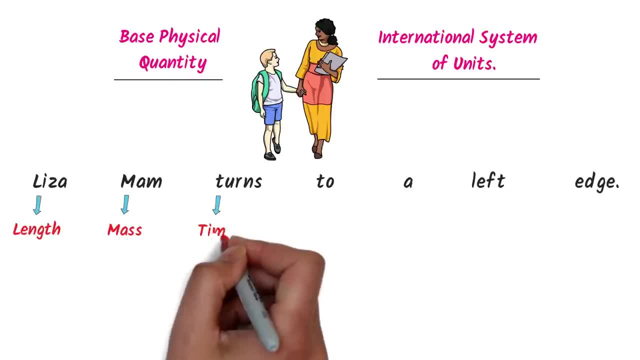 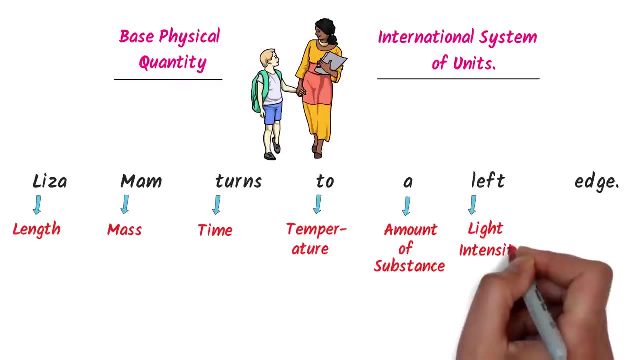 for length. M stands for mass. T stands for time. this T stands for temperature. S stands for amount of substance. L stands for light intensity. E stands for electric current. The SI unit of length is meter. The SI unit of mass is kg. 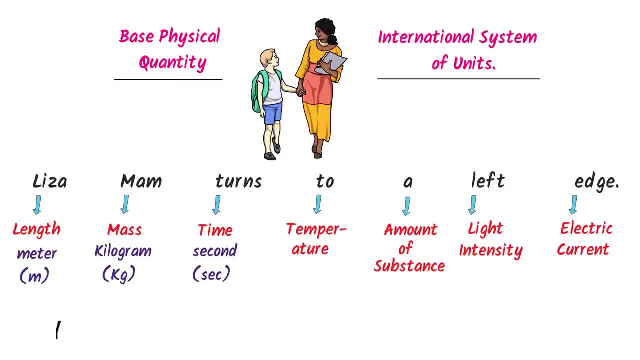 The SI unit of time is second, The SI unit of temperature is kelvin, The SI unit of amount of substance is mole, The SI unit of light intensity is candela And the SI unit of electric current is ampere. Remember that except these all seven units, the rest of units are called. 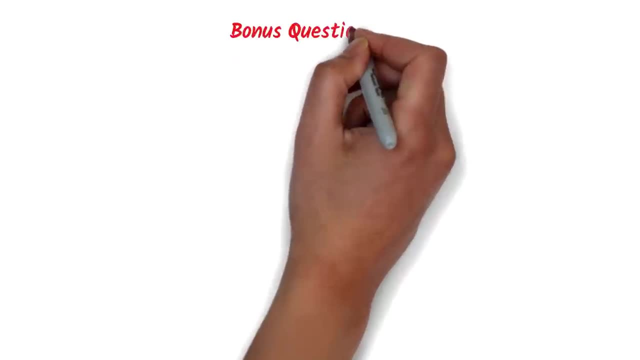 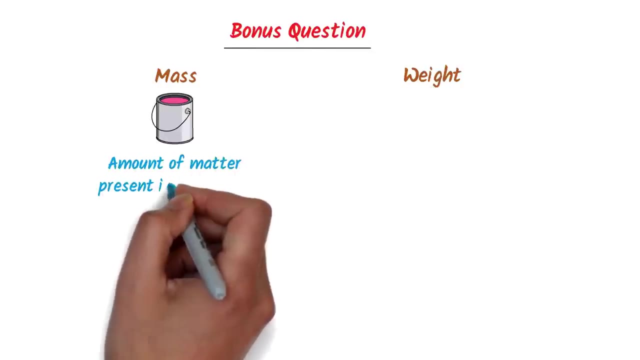 derived units. Also, let me teach you one bonus question: What is the difference between mass and weight? Well, mass is the force between the earth and an object. The SI unit of mass is kg and the SI unit of weight is Newton. So note it down, all these important points. 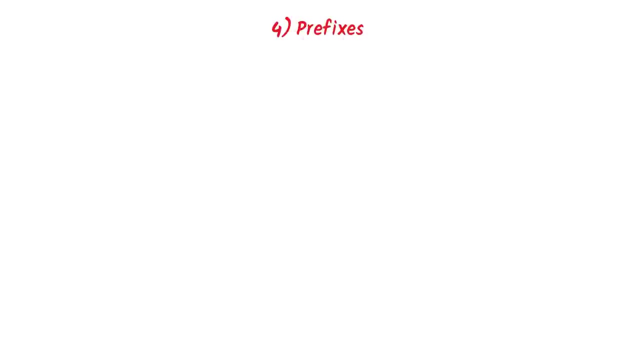 Now coming to the fourth topic. The fourth topic is about prefixes. A mnemonic that is added to units to show multiples or fractions are called prefixes. For example, consider two kilogram. Here gram is the unit and kilo is the prefix. Now how can we remember the? 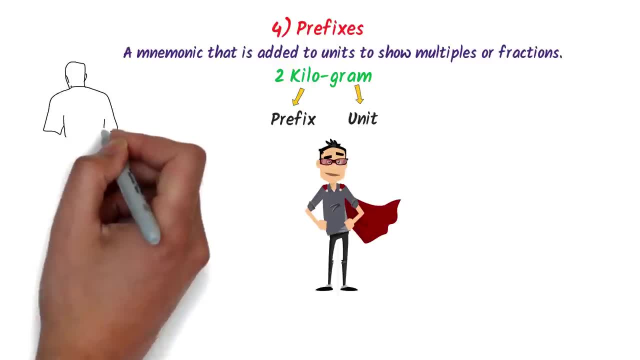 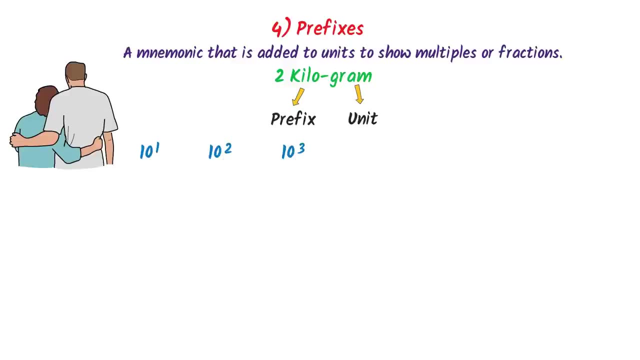 list of important prefixes. Well, I use my personal trick. I always write 10 to the power, 1,, 2,, 3, and then I jump three times: 6,, 9,, 12.. Now I say Dad has kept my great trick. 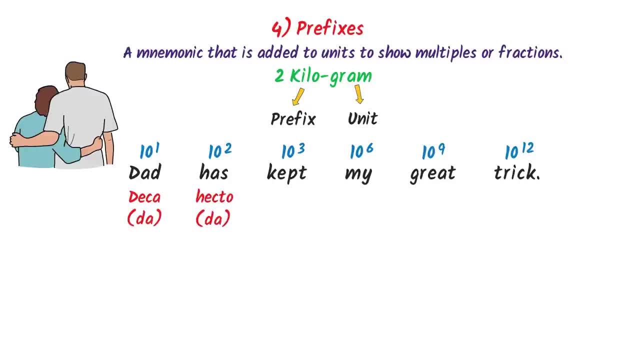 This D stands for deca, This H stands for hecto, This K stands for kilo, This M stands for mega, This G stands for giga And this T stands for tera. Secondly, I write 10 to the power, negative 1.. Then I write negative, 2, negative. 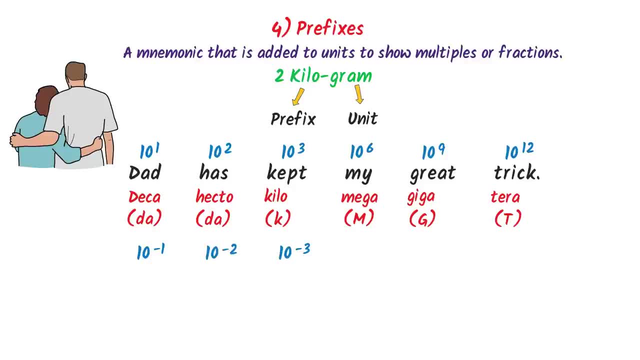 3. And then I repeat the previous process, jumping three times: Negative 6, negative 9, negative 12.. I use the trick- Dad can make me nice person Here. this D stands for deci. This C stands for centi. This M stands for milli. This M stands for micro. This N stands: 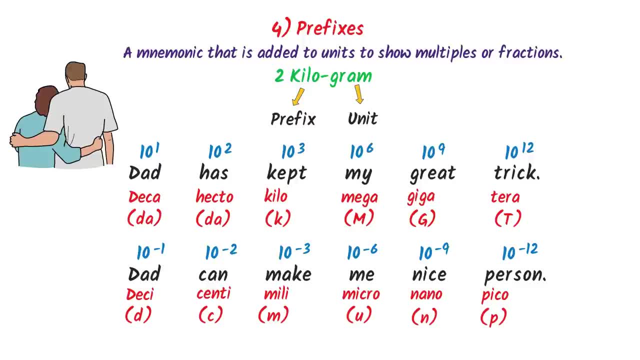 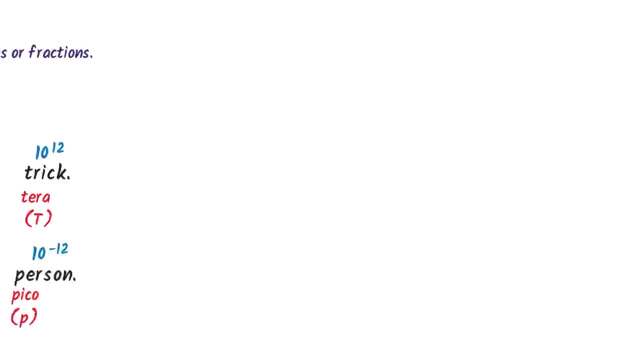 for nano. This P stands for pico. So this is the list of negative prefixes. Thus, using this trick, we can easily learn all the prefixes. The fifth topic is scientific notations. Well, a system of writing too big or too small numbers. 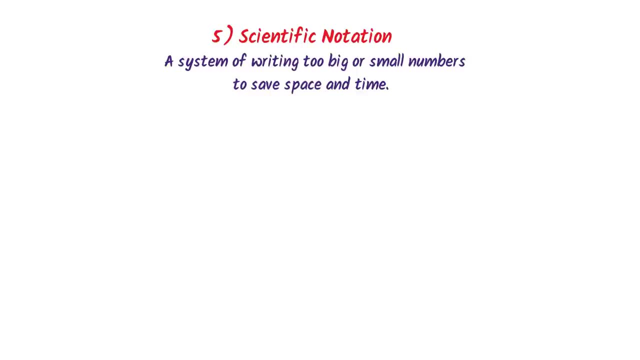 to save space and time is called scientific notation. For example, the mass of the earth is 6 into 10 to the power 24 kg. We can see that it is a very big number. So using scientific notation, we can easily save space and time. 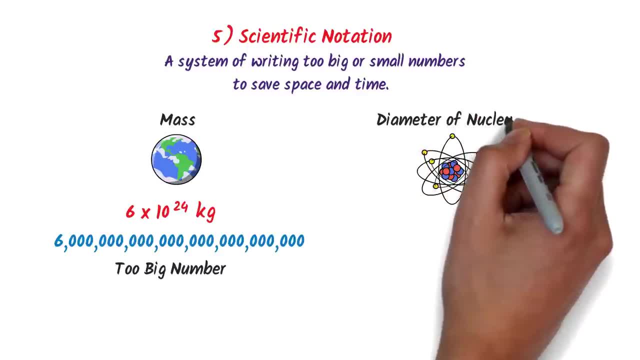 to write it. Also, the diameter of the nucleus is 1.7 into 10 to the power minus 15 meter, It is a very small number. So using scientific notation we can easily save space and time to write it. 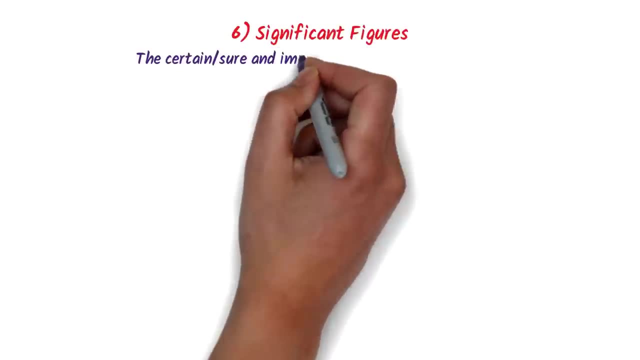 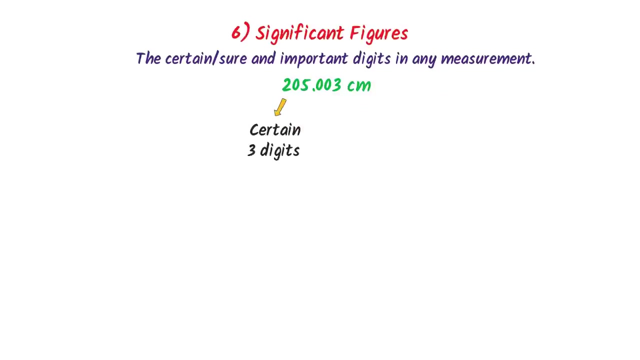 The seventh topic is significant figures. The certain are sure and important digits in any measurement are called significant figures. For example, consider this number: Here we know that 205 are certain are important 3 digits, While this 003 is uncertain. less. 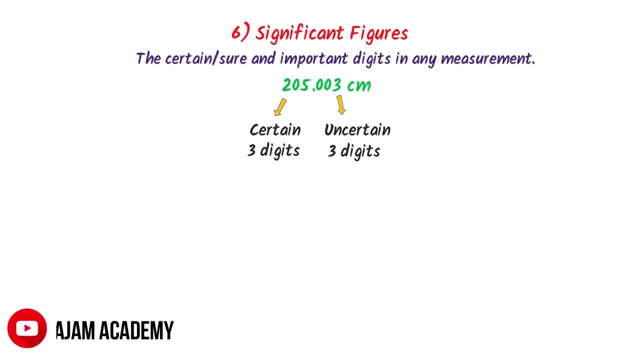 important 3 digits. So the collection of certain or less important digits are called significant figures. Now let me teach you the most simple trick to find significant figures. I write non-decimal numbers and decimal numbers, In case of non-decimal numbers, go from non-zero digit to last non-zero. 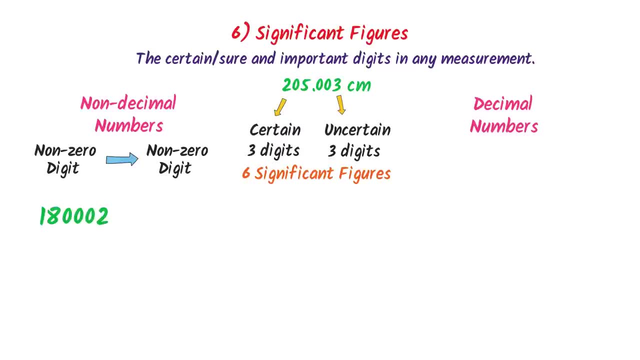 digit. For example, consider this number Here the first non-zero digit is 1 and the last non-zero digit is 2.. So I go from this 1 to this 2.. There are 6 digits in this number, So there are 6 significant figures. Similarly, consider: 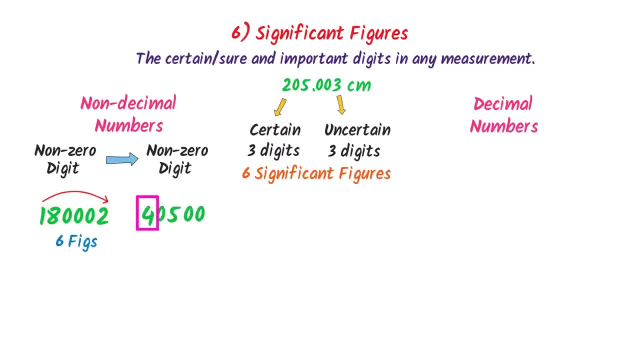 this number, The first non-zero digit is 4 and the last non-zero digit is 5.. I go from 4 to 5.. So there are 3 digits. I say there are 3 significant figures. Thirdly, consider this number Here: the first non-zero digit is 1 and the last non-zero. 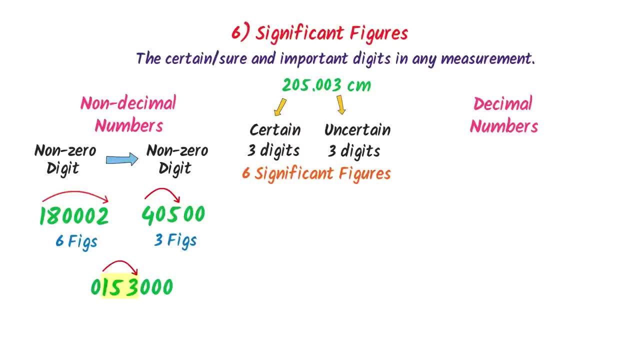 digit is 3.. So I go from 1 to 3.. There are 3 digits. I say there are 3 significant figures. Now, in case of decimal numbers, I go from first non-zero digit to last digit. For example: 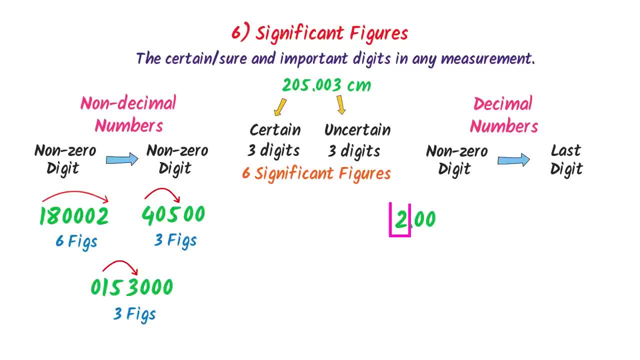 consider this number. Here the non-zero digit is 2 and the last digit is 0. So I go from 2 to 0. We can see that there are 3 digits in this number, So there are 3 significant figures. Secondly, consider this number. 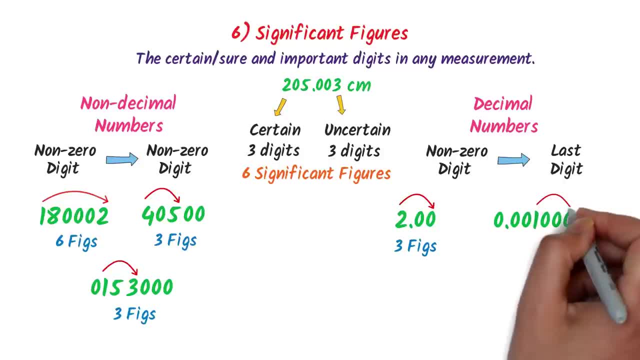 The first non-zero digit is 1.. So I go from 1 to the last. There are 4 digits, So there are 4 significant figures. Thirdly, consider this number. The first non-zero digit is 5.. So I go from 5 to the last. There are total 5 digits, So I say there are 5. 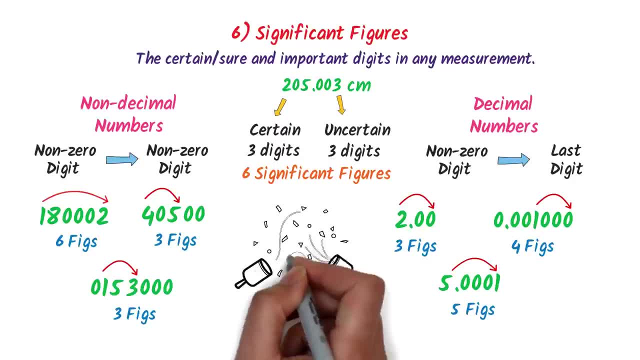 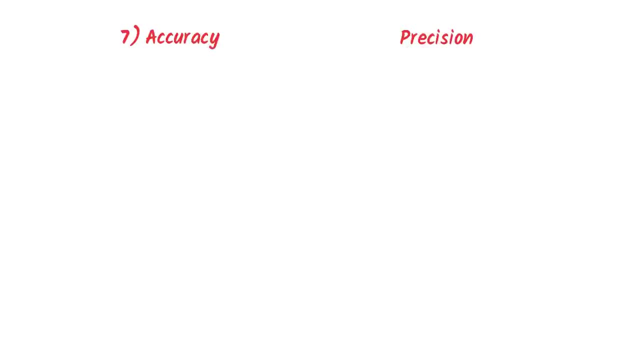 significant figures. Thus, using this simple trick, we can easily learn significant figures. The seventh topic is accuracy and precision. Accuracy means that how close you are to the actual value. For example, consider this man, Let the height of this man is 5 meter. Let. 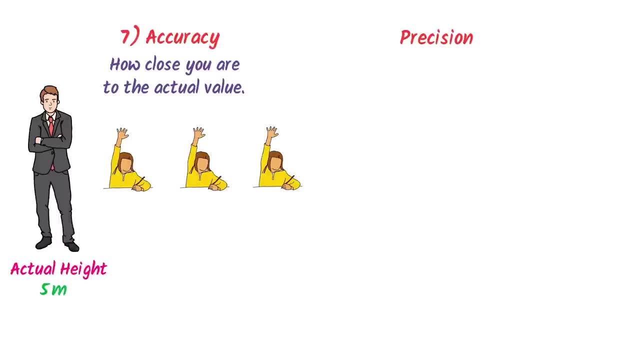 I ask 3 students to find the height of this man Let. the first student measured it as a 4 meter, The second student measured it as 4.5 meter And the third student measured it as 5 meter. Now these are the three different measurements. 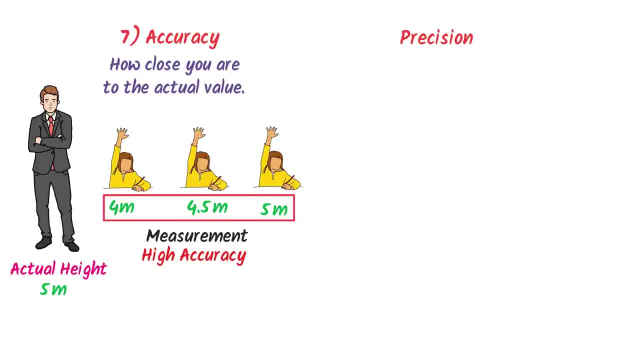 We say that this whole measurement is accurate result, Or we say that high accuracy Because the one measurement is exactly 5 meter, which is matching the actual height of the man. So the actual measurement is also 5 meter And this measurement of the student is also. 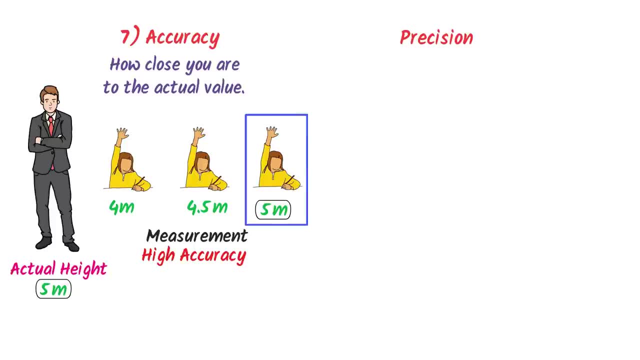 5 meter. So we say that this measurement is accurate or it has high accuracy. On the other hand, precision means that how does two or more measurements are close to each other? For example, consider the man from the previous example. We know that the 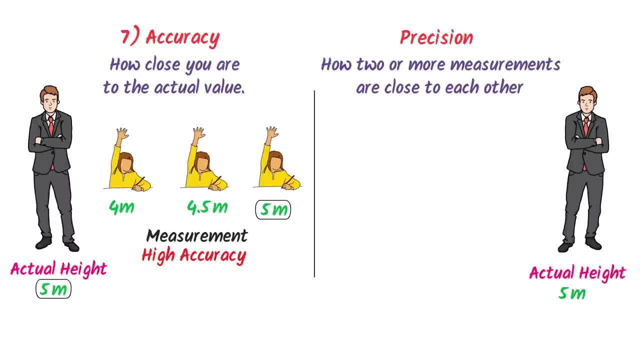 actual height of the man is 5 meter. Let I again ask three more students to find the height of this man. Let one student measured the height of this man as 3.5 meter, The second student also measured 3.5 meter And the third student measured it as 3.4 meter. 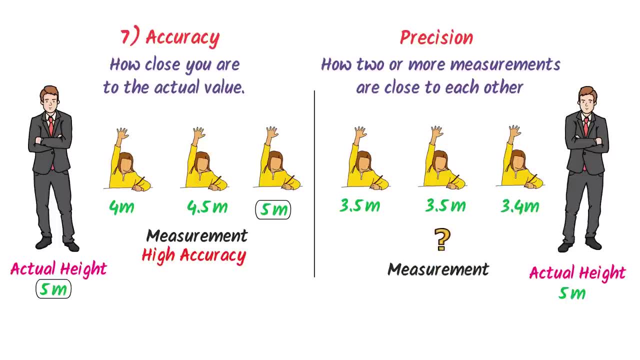 Now let me ask you: Are these three measurements are accurate? Your answer is no, Because the actual measurement is 5 meter and the measurements of the students are totally different from them. But wait a minute. Here we can see that this 3.5 and this 3.5 are close to each other, While this 3.5 and 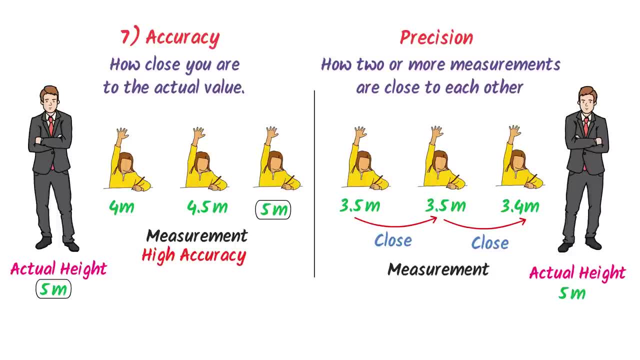 this 3.4 are also close to each other. The results of students are close to each other, So it has high precision. So we say that the first measurement of the student is close to the second measurement of the student and the second measurement of the students is close to the third measurement. 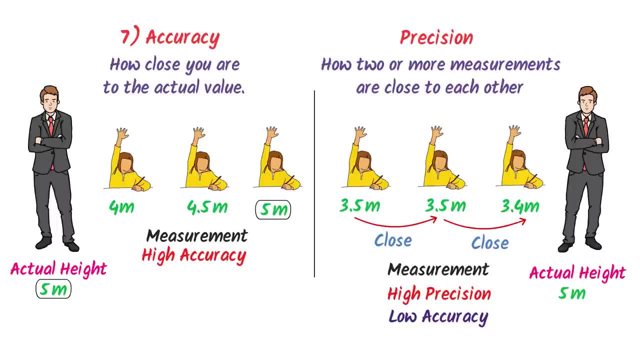 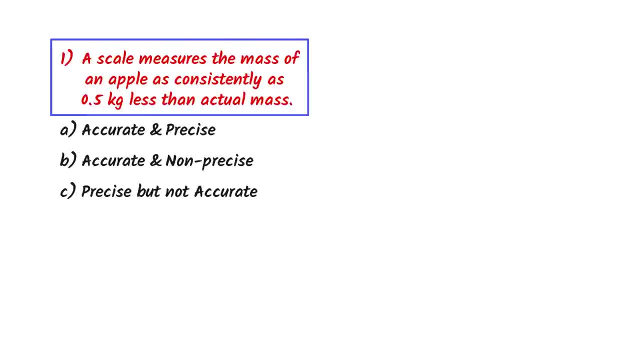 of the students. So we say that it has high precision. Thus, remember that it has high precision but low accuracy. Now let me teach you some important MCQs. A skill measures the mass of an apple as constantly as 0.5 kg less than the actual mass. 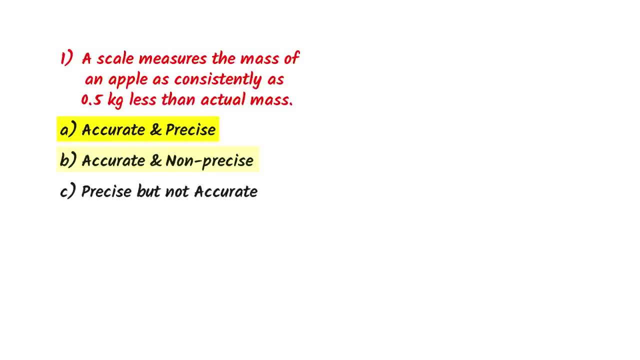 The options are accurate and precise, accurate and non-precise, precise but not accurate. Which one is right? Well, The C option is 100%. 0.5 is precise because the skill is constantly measuring 0.5 kg, 0.5 kg and 0.5 kg. 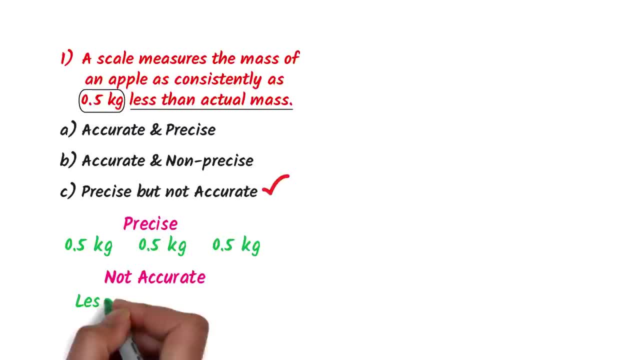 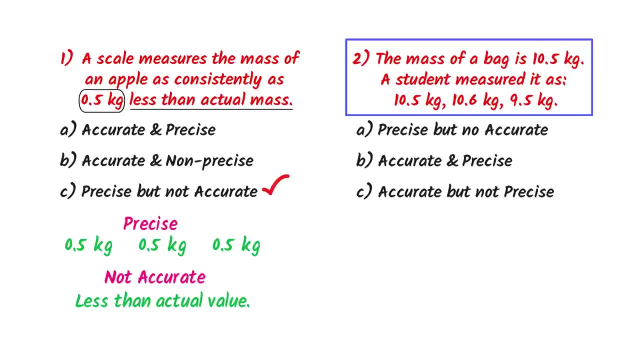 But this result is not accurate because it is less than the actual mass. The mass of a bag is 10.5 kg. A student measured it as 12.5 kg. 10.6 kg, 9.5 kg, 7.5 kg. 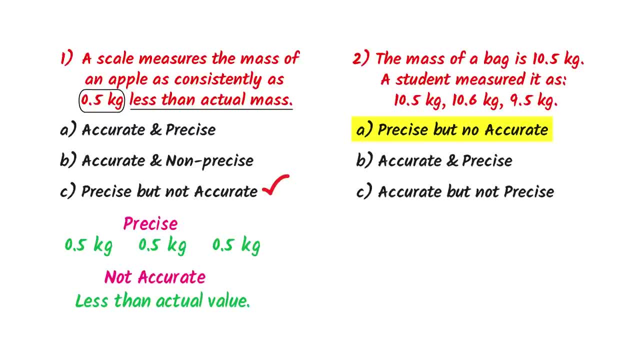 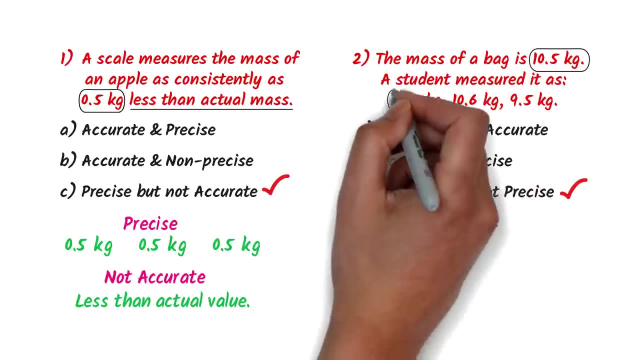 6.5 kg. The options are precise but not accurate. accurate and precise, accurate and not precise. Can you guess the correct option? Well, the correct option is C. It is accurate because one measurement of the student is matching the actual measurement. 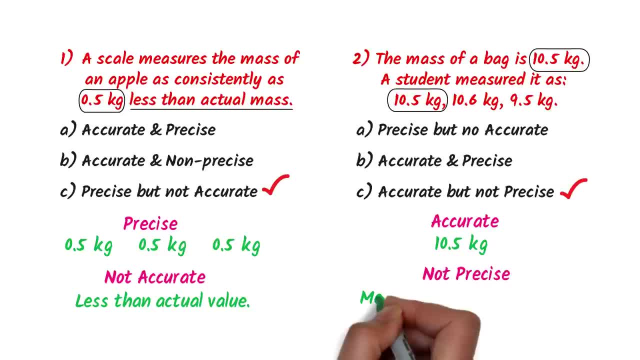 On the other hand, it is not precise because 9.5 kg is way different from 10.6 kg. Thus, this is all about accuracy and precision. Remember that we will not discuss topics of 9th class which we have already learned. 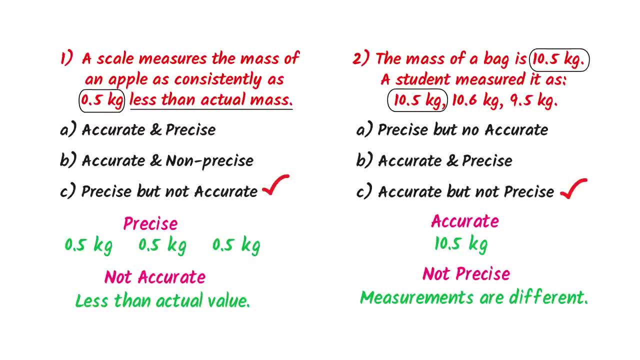 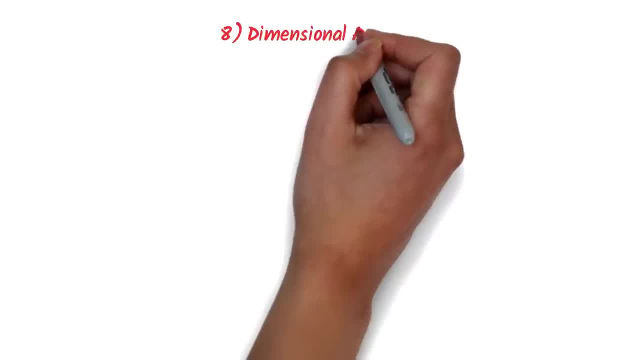 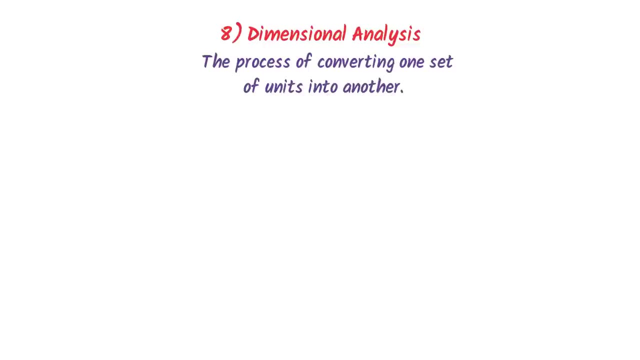 like atomic masses, relative atomic masses, atomic mass unit, percentage composition, etc. So the next important topic is dimensional analysis. The process of converting one set of units to another is called dimensional analysis. For example, Convert 3045 m to km and 35°C to kelvin. 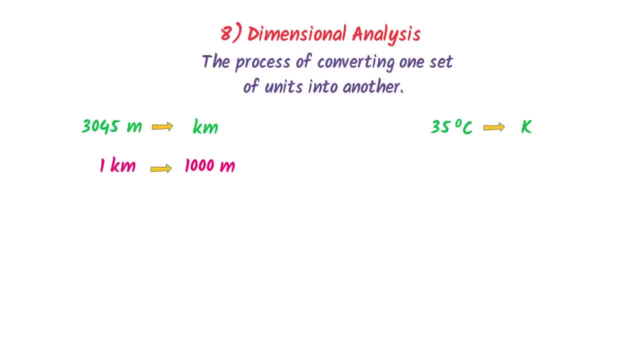 We know that in 1 km there are 1000 m. So I divide 3045 m by 1000.. I get 3.45 km. On the other hand, in 1°C there are 273 kelvin. 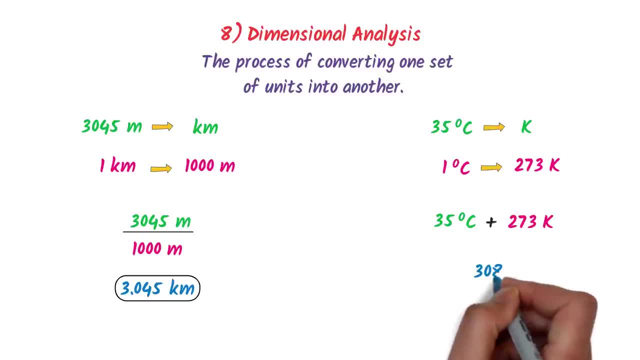 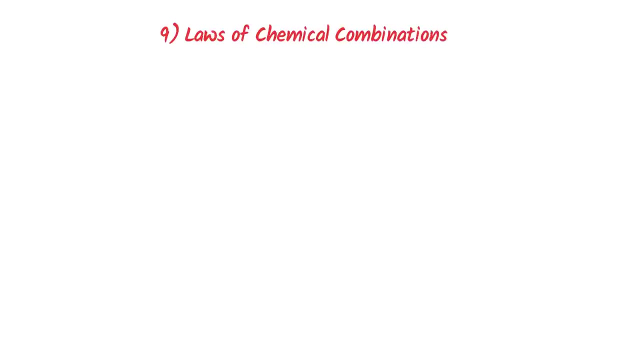 So 35 plus 273 is equal to 300 at kelvin. Thus this process of converting units from one set to another is called dimensional analysis. The 9th topic is laws of chemical combination. Well, there are 5 different laws or 5 subtopics that describe the basic rules by which atoms and molecules combine together. 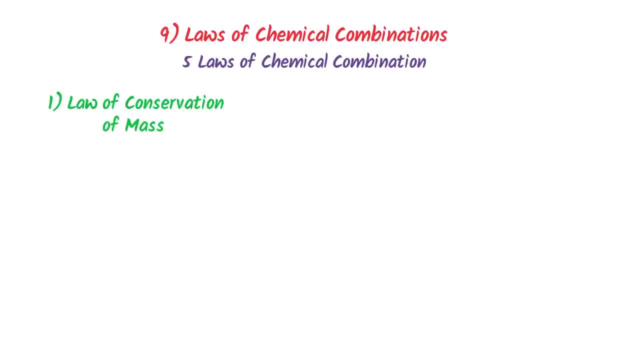 The first law is law of conservation of mass. Remember that it is all about the mass. It states that The mass of the reactants can neither be created nor destroyed in a chemical reaction. For example, consider 2 grams of hydrogen and 16 grams of oxygen. 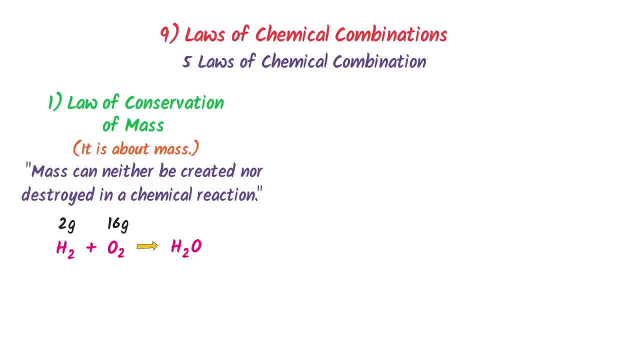 When they both react together, they form water. Now, if we measure the mass of the water, it would also be 18 grams. So we say that the mass of the reactants is 18 grams and the mass of the product is also 18 grams. 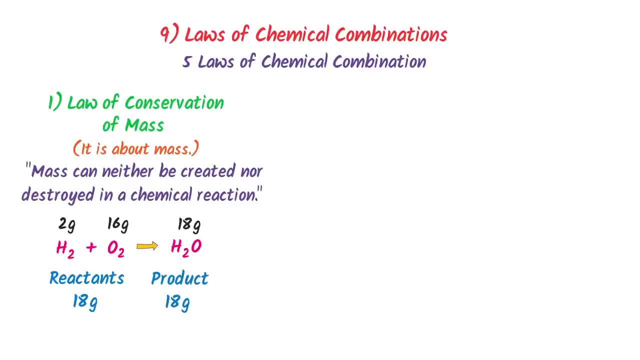 Thus they both are equal. That's why we say that. That's why we say that mass can neither be created nor destroyed in any chemical reaction. The second law is law of definite proportion. Remember that it is based on ratio of masses. 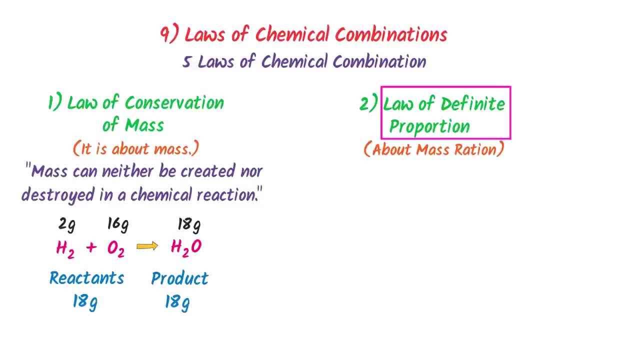 The word definite proportion means fixed amount. It states that It states that chemical substances are made up of elements that are present in fixed ratio by mass. For example, consider water and hydrogen peroxide. In water, the ratio of hydrogen to oxygen is 2 to 1, while in hydrogen peroxide the ratio of 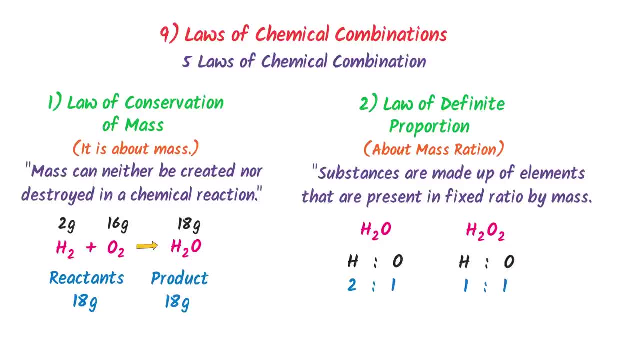 hydrogen to oxygen is 1 to 1.. It shows that the ratio of oxygen and hydrogen would always be 2 to 1 and the water, while the ratio of hydrogen and oxygen in hydrogen peroxide would always be 1 to 1.. Therefore we say that chemical substances combine in fixed ratio by mass. The third law: 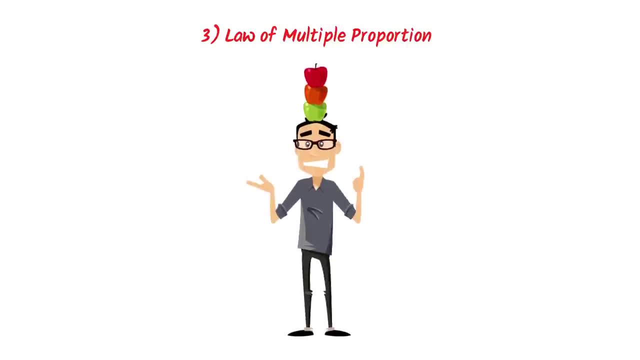 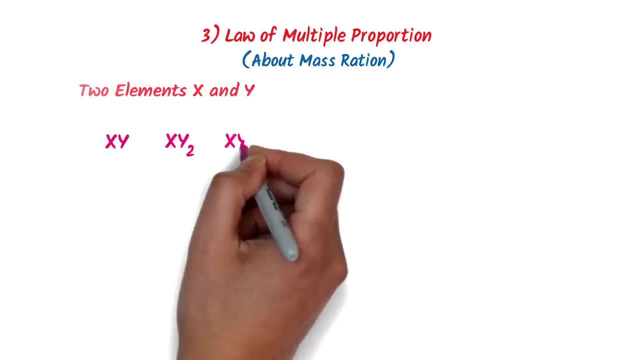 is law of multiple proportion. It is very difficult for students, but I will crack it. It is also based on ratio of mass. Now consider two elements like x and y. Let they form three different compounds: xy, xy2, xy3.. Now we can see that the ratio of x and all these 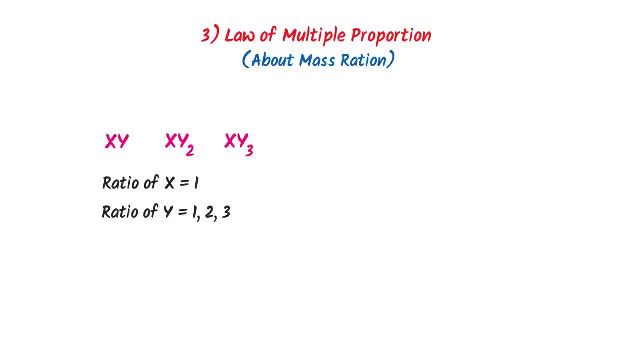 things are 1 to 1.. Therefore we say that chemical substances combine in fixed ratio by mass. The ratio of x and all these three compounds is 1,, while the ratio of y in all these three compounds is 1,, 2 and 3.. Now listen carefully. We say that if y combine with the same element, x, 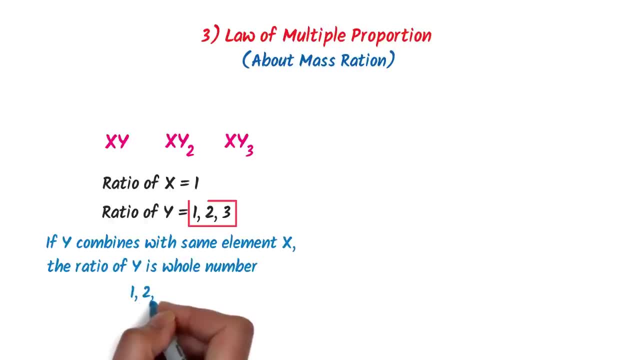 the ratio of y is whole number like 1,, 2, 3.. Let me repeat it: If y combine with the same element, x, the ratio of y is the whole number like 1,, 2, 3.. This is what the law of multiple proportion. 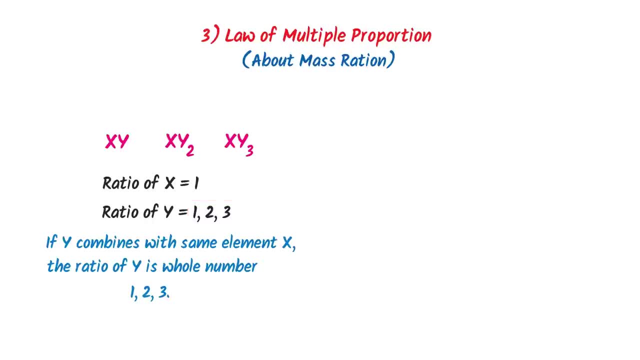 explains. Let me give you one real example. Consider carbon monoxide and carbon dioxide. In carbon monoxide, the ratio of masses is 12 to 16, while in carbon dioxide the ratio of masses are 12 to 32.. Now dividing this whole thing by 12.. 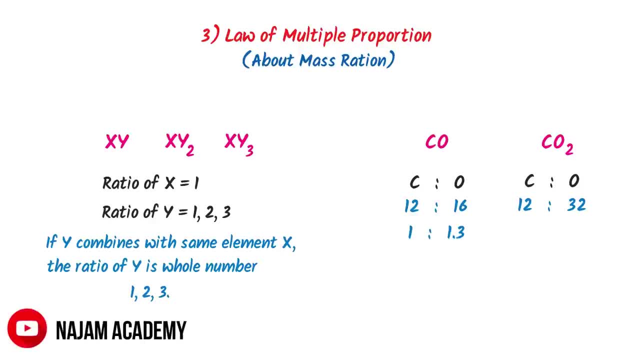 In carbon monoxide the ratio of carbon is 1 to 1.3,, while in carbon dioxide the ratio of carbon is 1 to 1.3.. is 1 to 2.. So the ratio of carbon is 1 in both the compounds, but the ratio of oxygen. 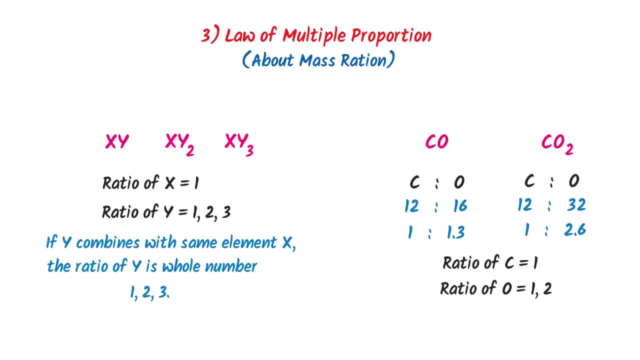 is 1 to, which is again whole number. Therefore, this law states that when two elements like x and y form two different compounds, the ratio of the mass of y can be expressed as whole numbers. So this is what the law of multiple proportion teaches. 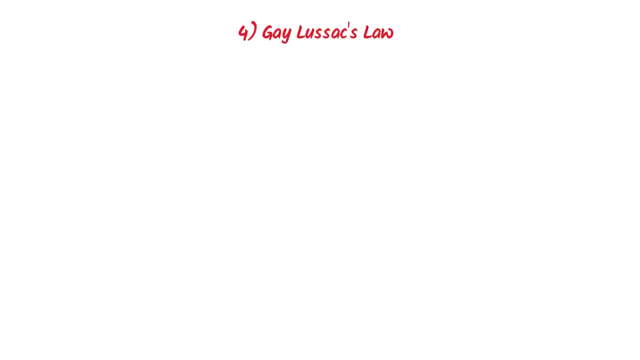 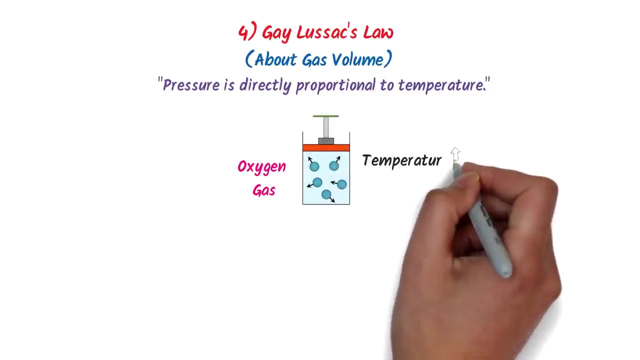 The fourth law is Gay-Lussac's law. Remember that it is based on volume of gases. It states that pressure is directly proportional to temperature. For example, consider oxygen gas and this cylinder. If we increase the temperature of the gas, the rate of collision. 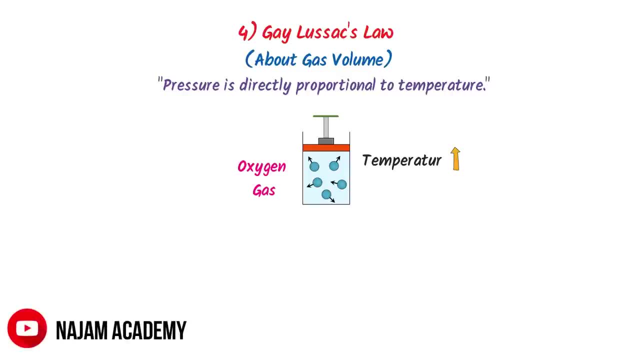 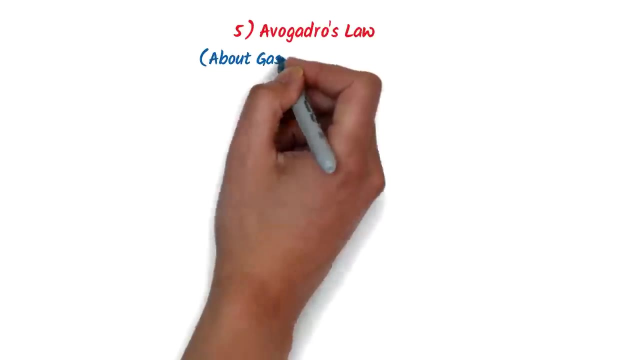 of oxygen molecules on the wall of container is increased. As a result of this, pressure is increased. So we say that pressure is directly proportional to temperature. The fifth law is Avogadro's law. Remember that this law is based on volume and mass of a gas. It states that volume is directly. 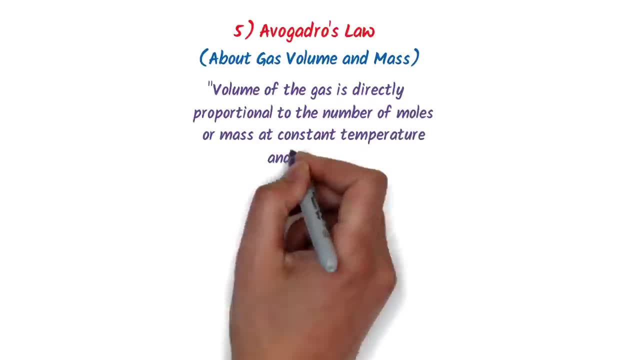 proportional to number of moles or mass of the gas at constant temperature and pressure. For example, consider these balloons. As you fill these balloons with more air or more mass, their volume increases. The fifth law is Avogadro's law. Remember that this law is based on volume and mass. 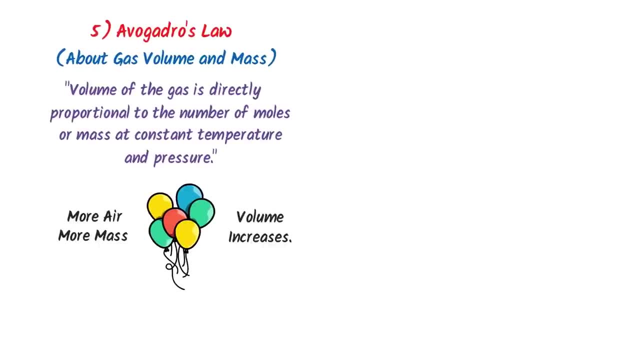 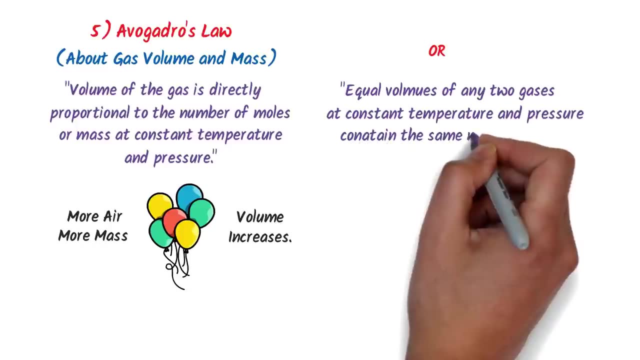 of a gas. So if we increase the temperature of cells, as discussed earlier, pressure increases. The fourth law is Gay-Lussac's law. Remember that we can also write Avogadro's law- as equal volumes of any two gases at constant temperature and pressure contains the same. 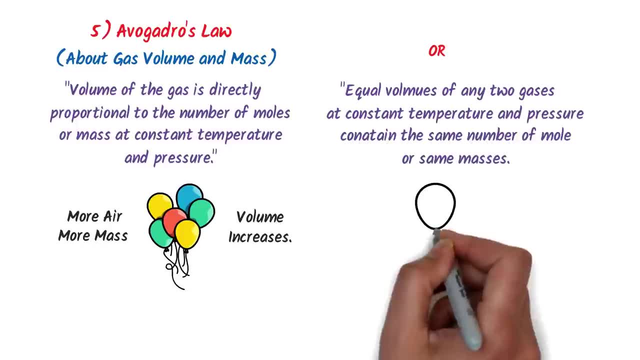 number of moles or same masses. For example, consider 2でも cube hydrogen gas and 2 dzm cube of oxygen gas Let they both are present at constant temperature and pressure. So we say that they both contain equal number of molecules. 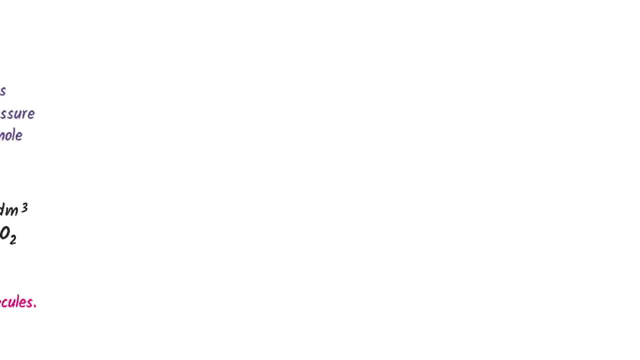 to snotter down these laws of chemical combinations. The tenth topic is mole and Avogadro's number. In our daily life we say that one dozen egg is equal to 12. So we say that one dozen is nothing but just like a number. 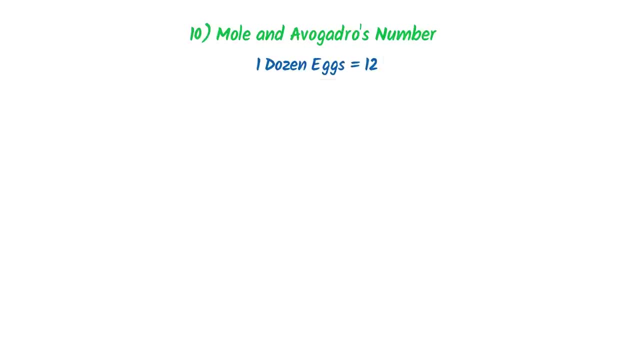 Now to learn the concept of mole and Avogadro's number, we should learn relative atomic mass and molar mass. For example, the relative atomic mass of carbon is 12 amu. Remember that there is only one atom of carbon present. 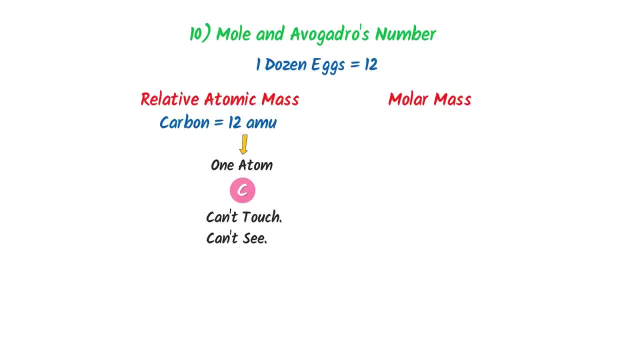 Now, we cannot touch, we cannot see and we cannot do chemistry with one atom of carbon. To solve this issue, scientists put forward the idea of molar mass. Now, instead of 12 amu, if I take 12 grams of carbon, it is known as a molar mass. 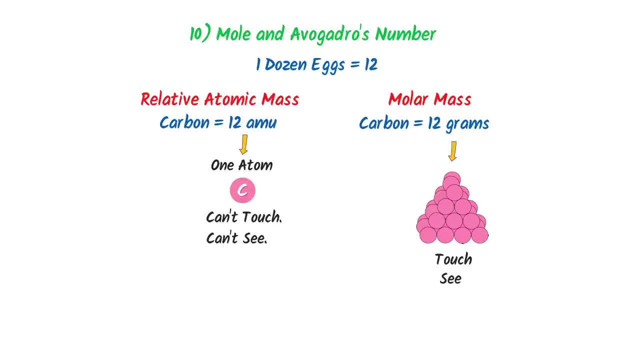 Remember that we can touch, we can see, we can do chemistry with molar mass of carbon. We know that at 12 amu there is only one atom of carbon, but at 12 grams there are total 6.023 x 10 to the power, 23 atoms. 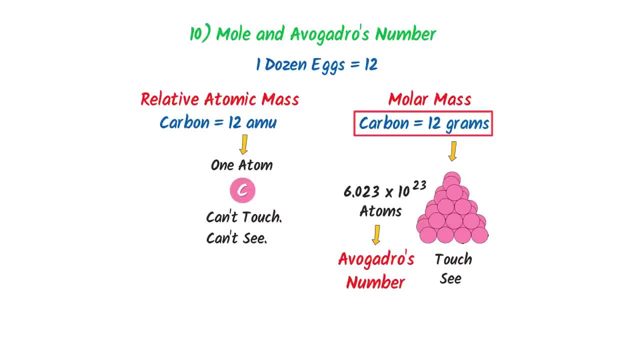 Thus this number is known as Avogadro's number. Thus, remember that at 12 grams of carbon, there are 6.023 x 10 to the power, 23 atoms. Now listen carefully: One mole is always equal to one atom of carbon. 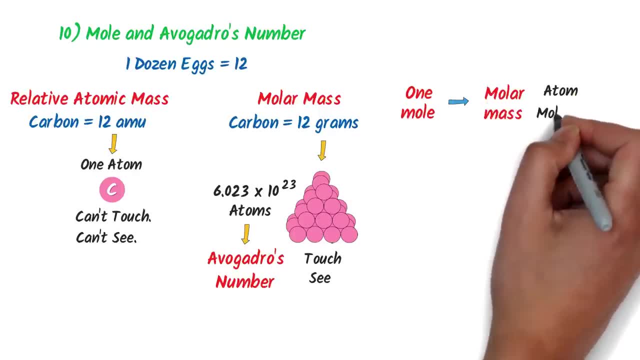 Now listen carefully. One mole is always equal to molar mass of an atom, molecule or formula unit. Also, we know that molar mass of any atom, like carbon, molar mass of any molecule and molar mass of any formula unit contain 6.023 x 10 to the power 23 atoms. 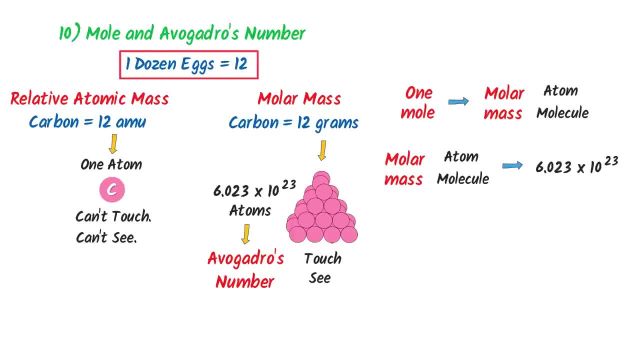 So remember that one dozen of anything is always equal to 12.. One mole or molar mass of any atom molecule or formula unit contain 6.023 x 10 to the power 23 atoms. So remember that this is used to calculate molar mass of an atom. 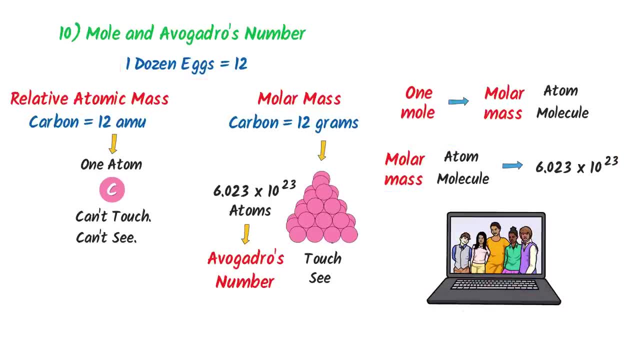 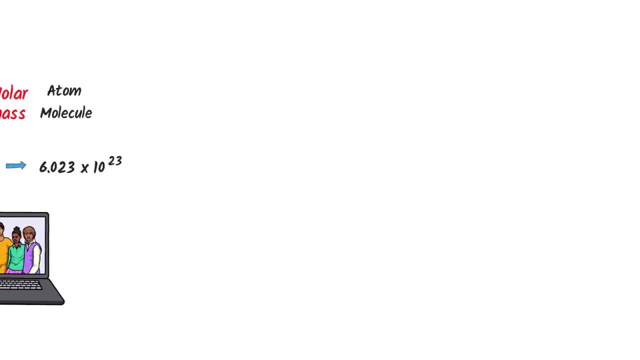 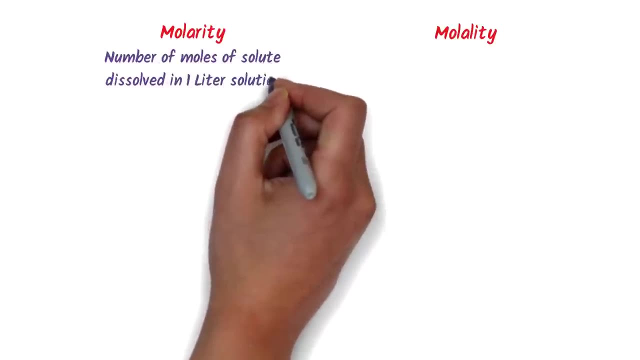 If you want to learn more about mole concept and Avogadro's number, we have already uploaded a very dedicated video and its link is given in the description. Now the last topic is molarity and molality. Now, molarity is the number of moles of solute dissolved and 1 liter solution. 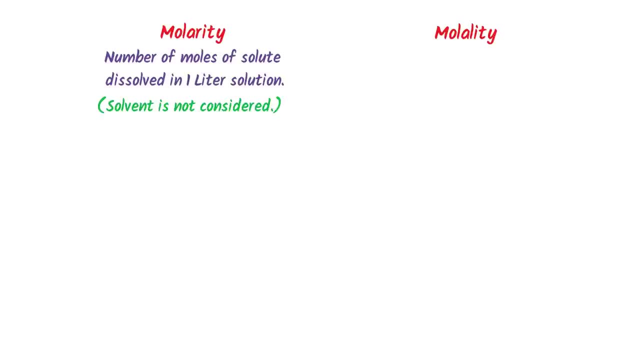 Remember that we do not consider solvent and molarity. For example, consider some water and this object. I add 2 moles sugar to this water. After adding 2 moles sugar to this water, the volumes of solution becomes 1 liter.